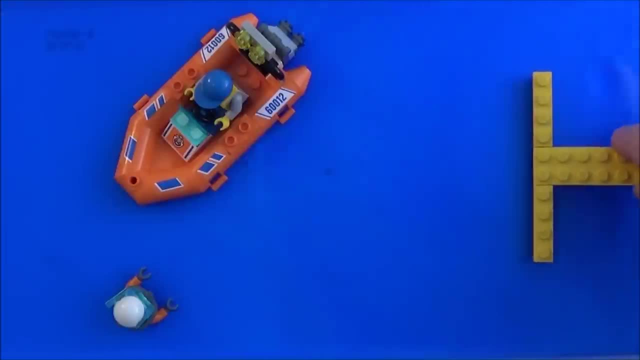 they move. We can think about plane waves, which may be made by this rather large dibber, so it's fairly long at the front. We can also think about having a point source of waves. This is a bit like if you throw a stone into a pond and what we get then are ripples moving. 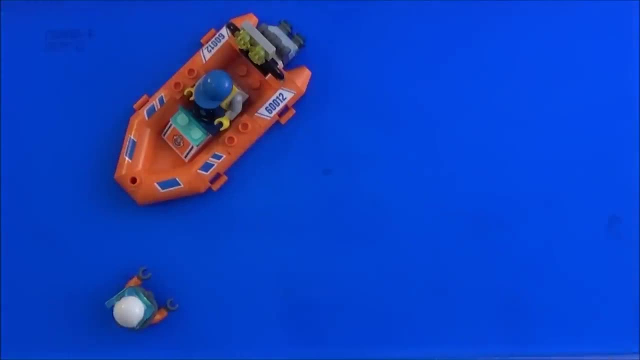 off a circular path. However, as you can see, it's not that easy to show the ripple tank. The ones at school are fairly big and you do see the effect, but it's not always that clear. So you need to know about a real ripple tank and how it's set up. but we can. 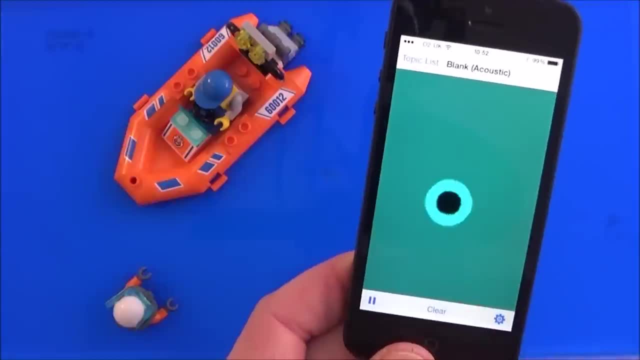 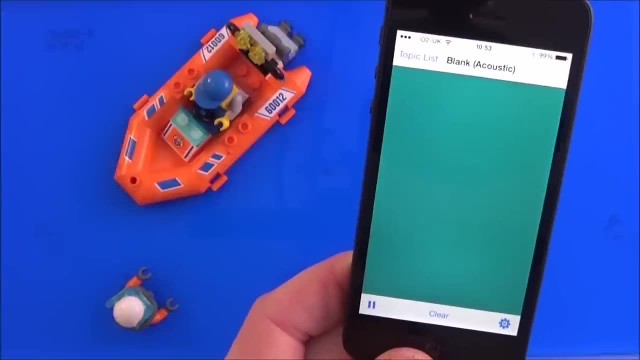 also model this using this rather nice app on the phone. The details are in the link below. What we can do is we can send out ripples. we can look at different effects and some of the basic wave properties, both for electromagnetic and mechanical waves. 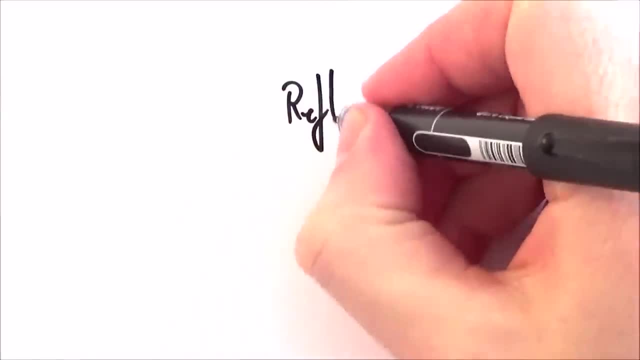 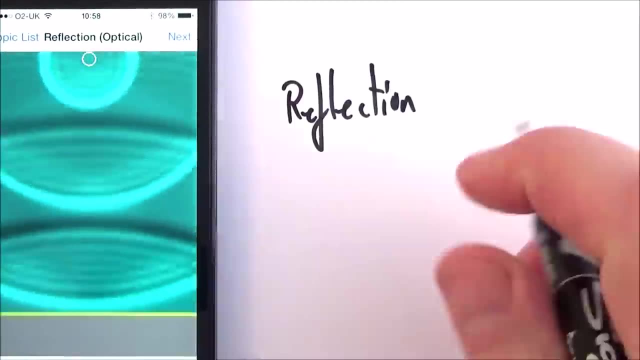 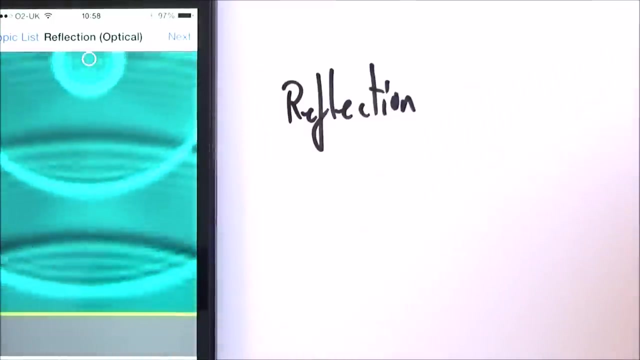 There are a few properties I'd really like to look at, and these include the reflection of waves, which is when the wave hits another surface and bounces off. In terms of light, we see this effect a lot with a mirror, and in terms of sound, we know this as an echo. 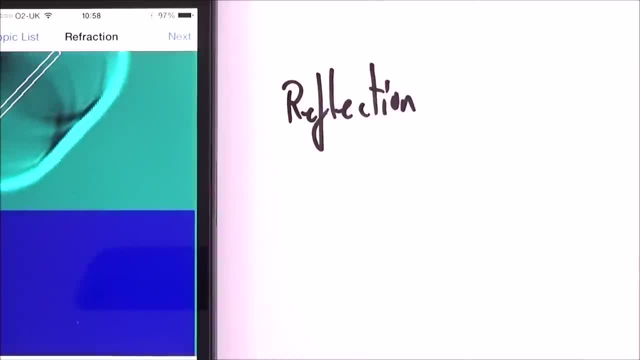 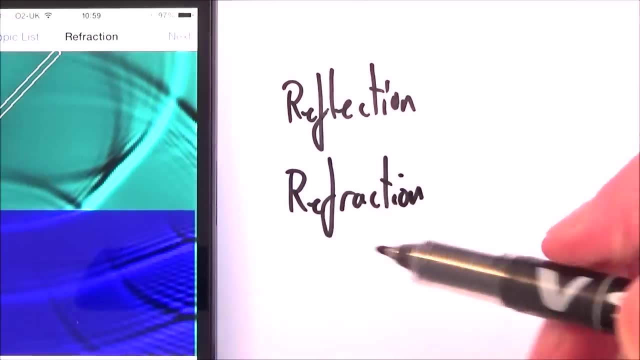 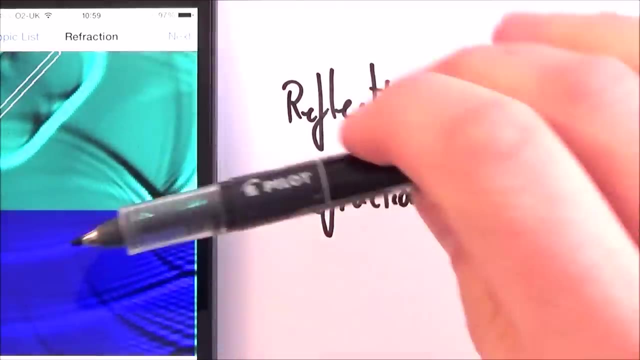 So that's reflection of waves. We also have refraction, So refraction is where a wave changes direction as it moves from one medium into another, which is a different kind of density. So what we have here are the wave fronts. These are positions at the front of. 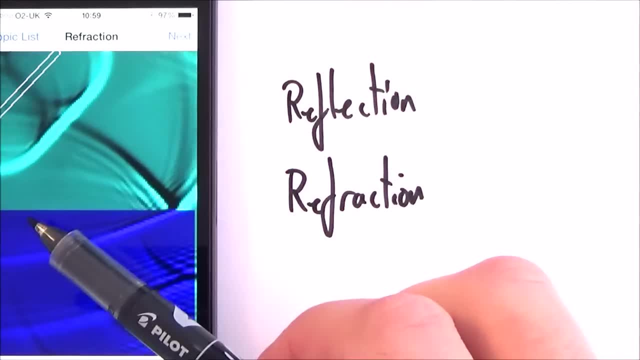 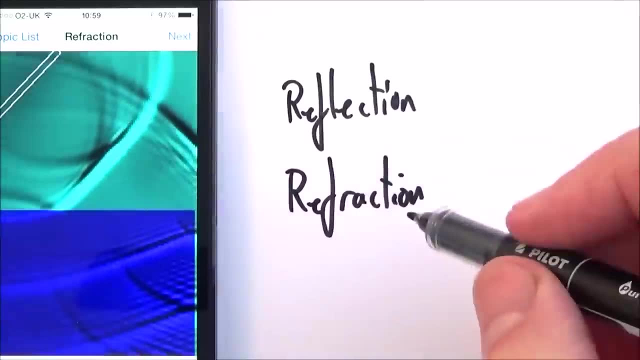 a wave. We've got a nice plain wave front. As it comes along, you can see that one side of that wave front hits the other medium before the other and it bends away. And again I've got another video which will be all about refraction and some of the effects. 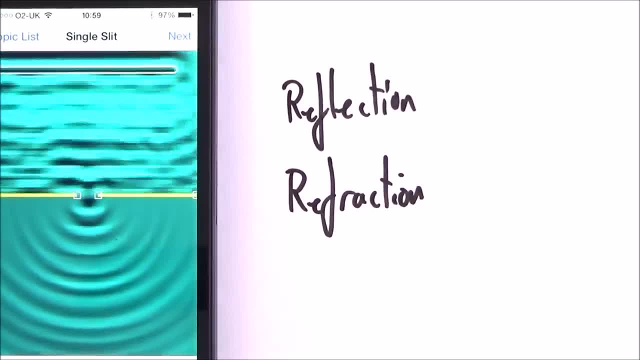 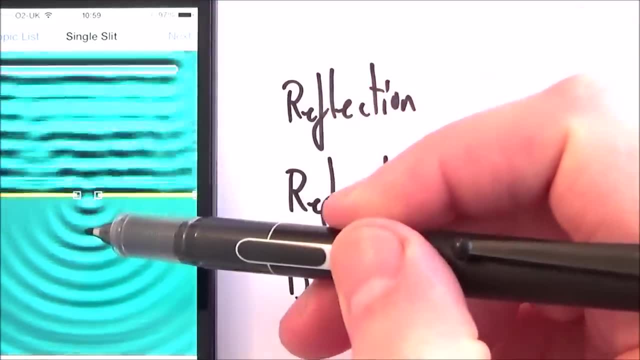 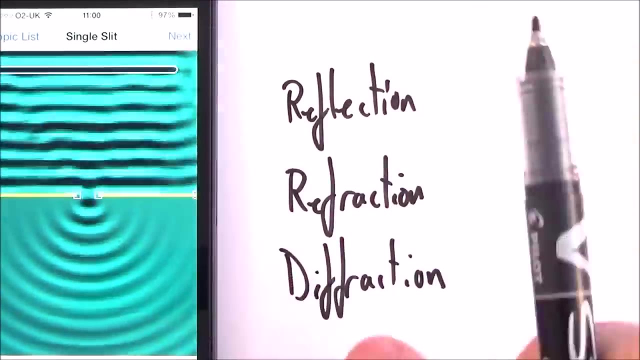 when we look at Snell's Law and so on, We also have an effect called diffraction. So diffraction is when a wave moves through a gap and what we see is, if the wavelength is approximately equal to the gap size, the wave tends to spread out in all directions. 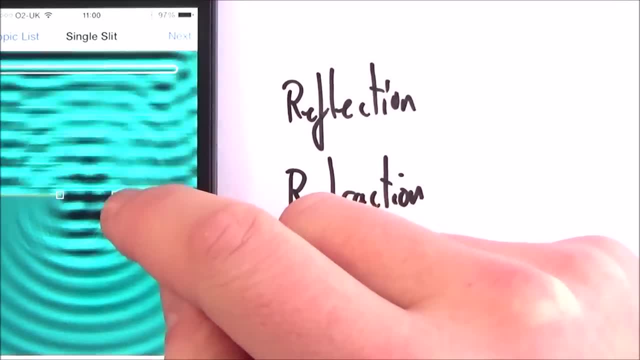 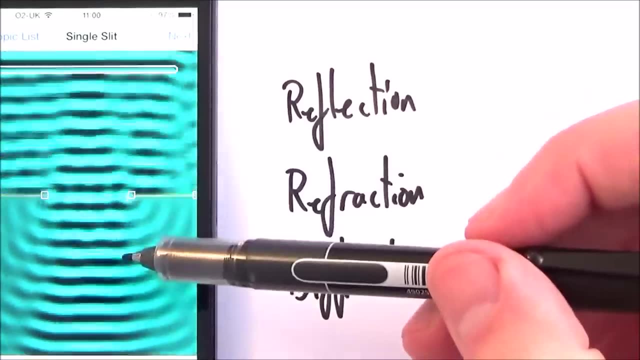 The great thing about this app is that you can do loads of things. You can change the frequency, You can change the wavelength. If I make that gap a little bit wider- so now the gap is a lot wider than the wavelength- then the waves don't spread out as much, And this is